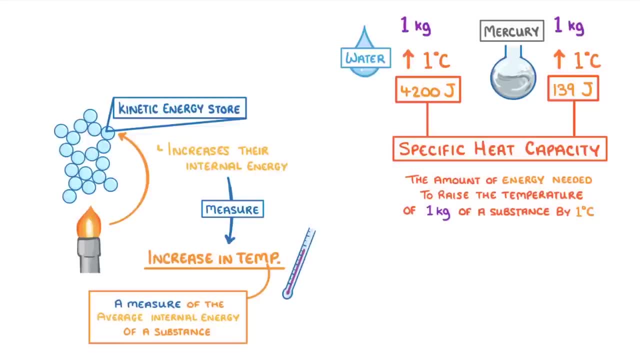 of energy needed to raise the temperature of 1 kilo of a substance by 1 degree Celsius. It can also be thought of as the amount of energy released as that substance cools. So each time our kilo of water cools by 1 degree Celsius, it will give out 4200 joules. 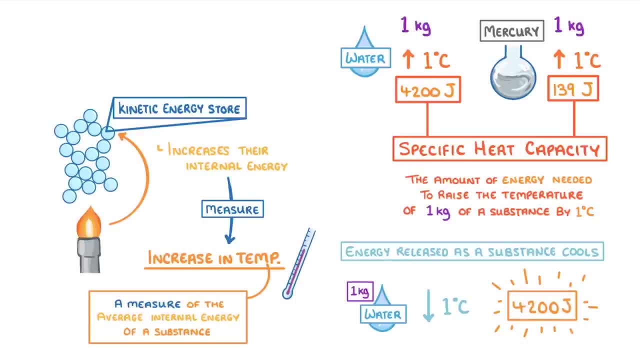 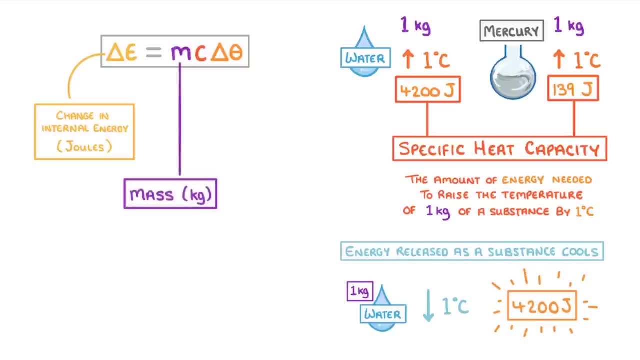 of energy to the surroundings. We can put this idea into an equation where the change in internal energy is equal to the mass times, the specific heat capacity for that particular substance. So we have the temperature times, the change in temperature, With the triangles meaning. 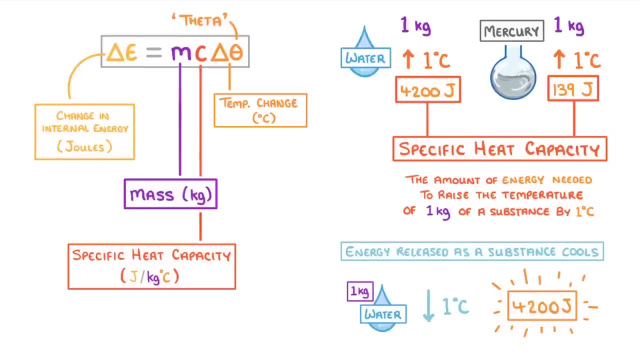 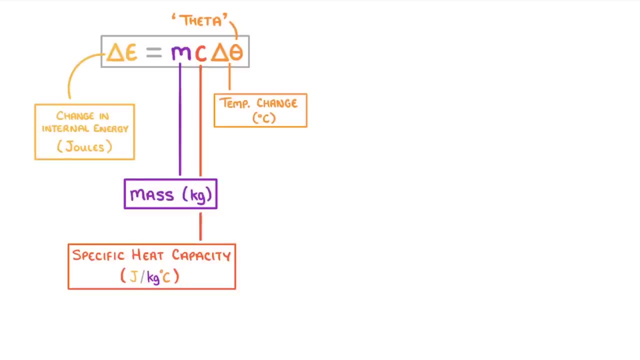 change and the 0, the line through it being a theta sign, which here means temperature. To see how this works, let's try a question. Find the final temperature of 800g of water at an initial temperature of 20 degrees Celsius after 20 kilojoules of energy has been transferred. 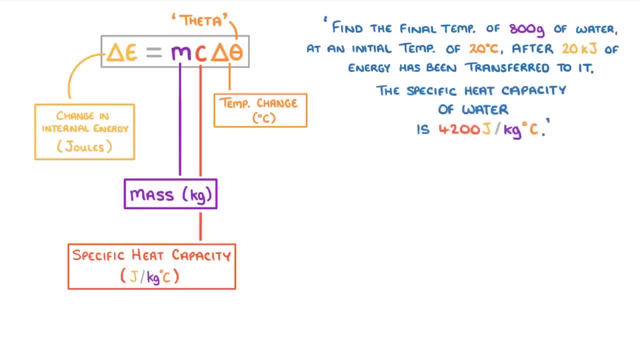 to it. The specific heat capacity of water is 4200 joules of water. In order to find the final temperature, what we're really looking for is the change in temperature, So to get that term by itself, we need to divide both sides by mc, giving us energy. 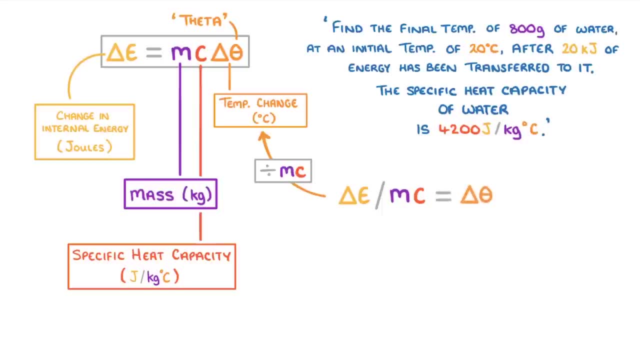 divided by mass times. specific heat capacity equals change in temperature. Next, we make sure all of our units are correct. So change 800g to 0.8 kilos and change 20 kilojoules to 20,000 joules and then plug. 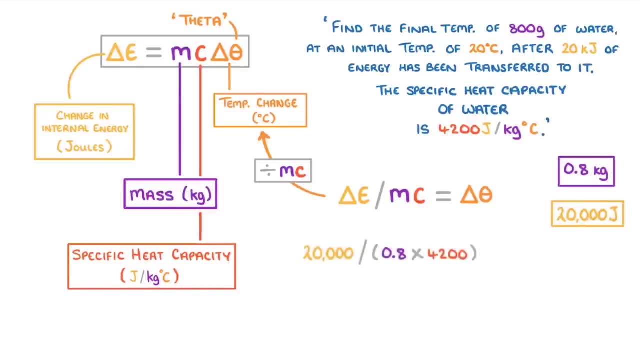 these values into the equation. So overall we get a temperature change of 5.95 degrees And if we add that onto our original 20 degrees, the final temperature would be 25.95 degrees or 26.0 degrees. 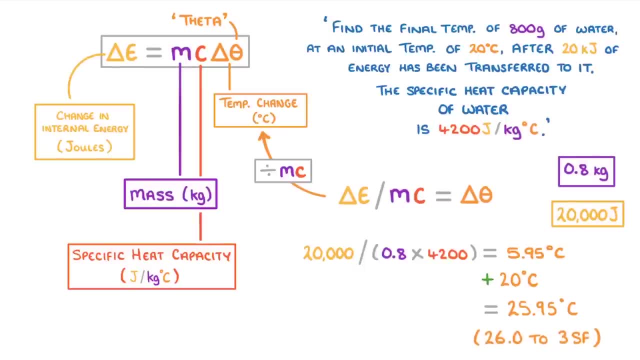 If we round it to three significant figures, which we generally should. One thing to point out here is that in real life, the temperature probably wouldn't actually increase this much, because some of the energy would be lost to the surroundings, mostly in the form of heat.